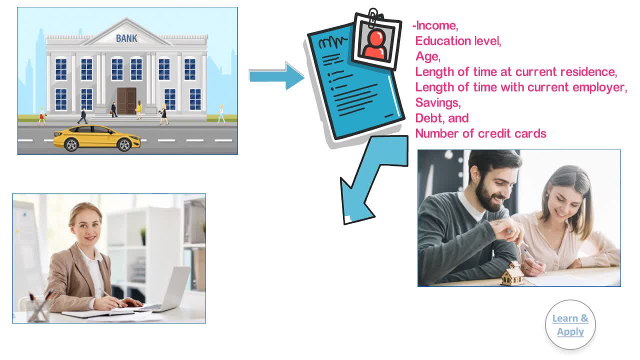 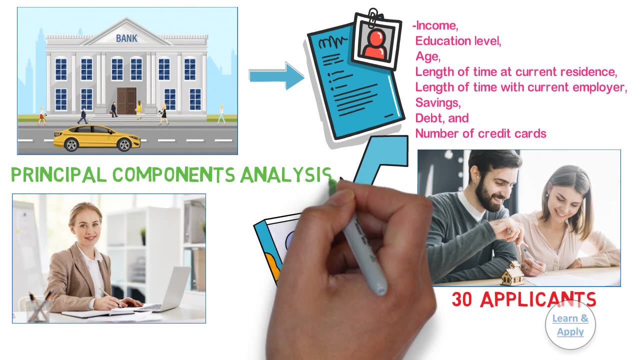 A bank administrator wants to analyze this data to determine the best way to group and report. The administrator collects this information for 30 loan applicants. Here the administrator performs a principal component analysis to reduce the number of variables, to make the data easier to analyze. 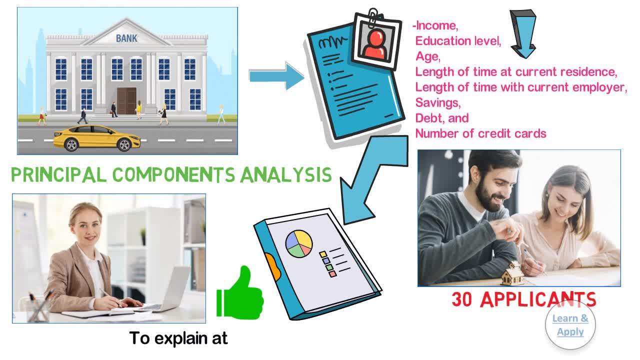 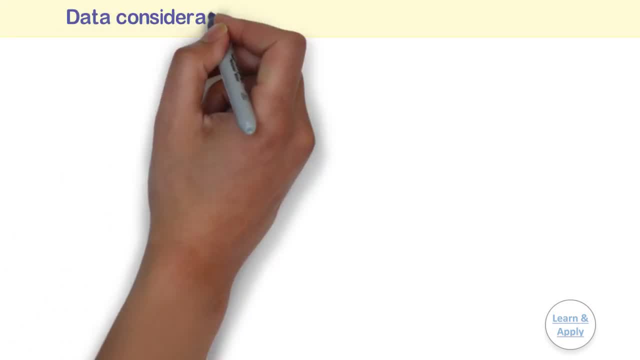 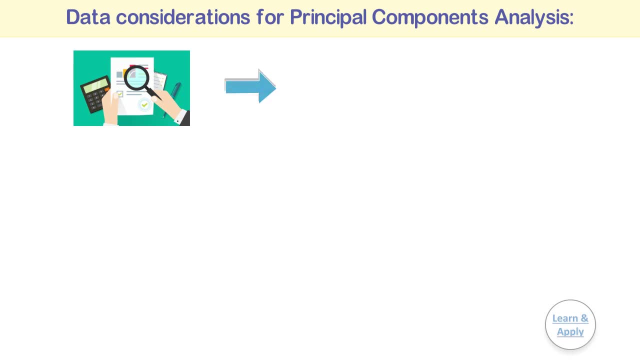 The administrator wants enough components to explain at least 90% of the variation in the data. Data considerations for principal component analysis. To ensure that your results are valuable, consider the following guidelines when you collect the data, perform the analysis and interpret your results. 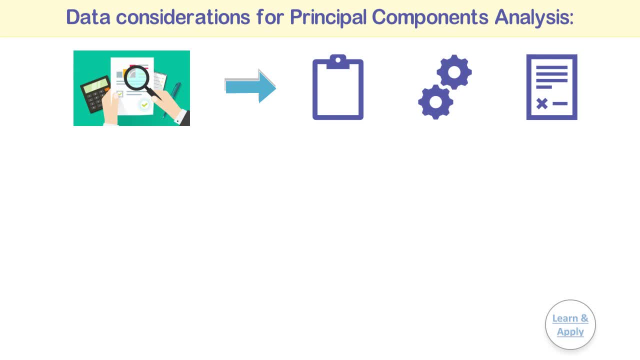 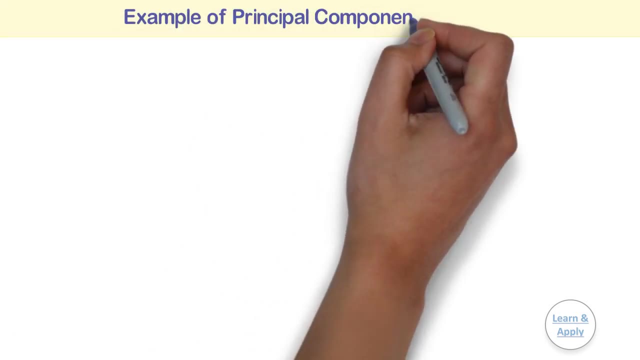 In the case of principal component analysis, there is only one requirement of data, and that is: you should have at least two variables, and the measurements for each variable should be recorded in separate numeric columns. Example of principal component analysis. Let's continue with the same example. 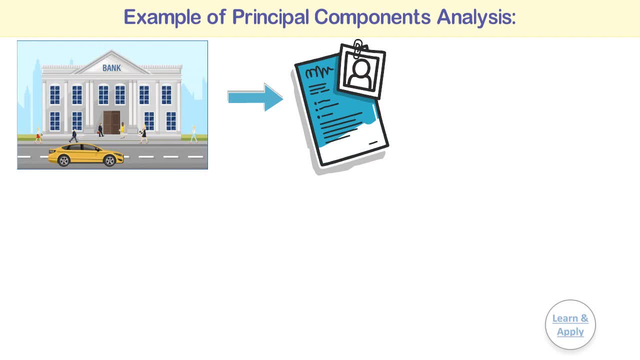 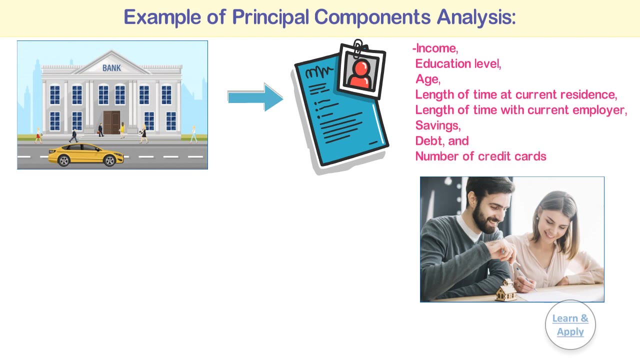 A bank requires eight sections of information from loan applicants, like income, education level, age, length of time at current residence, length of time with the current employer, savings debt and the number of credit cards. A bank administrator wants to analyze this data to determine the best way to group and report it. 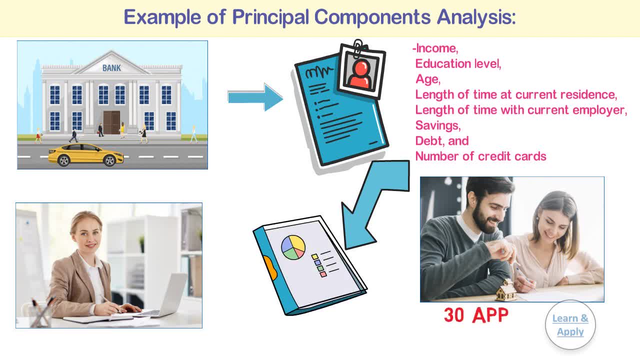 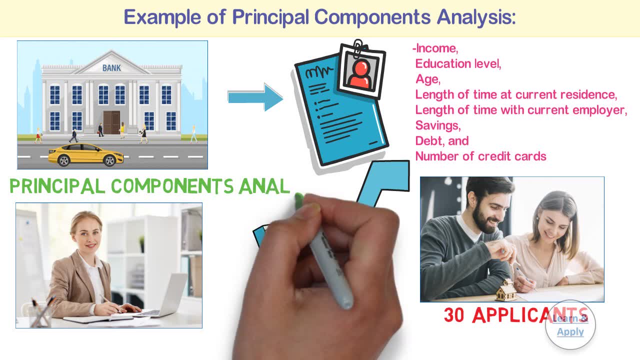 The administrator collects this information for 30 loan applicants. Here the administrator performs a principal component analysis to reduce the number of variables, to make the data easier to analyze. The administrator wants enough components to explain at least 90% of the variation in the data. 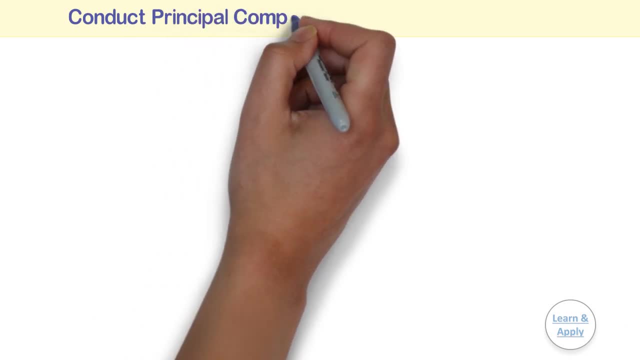 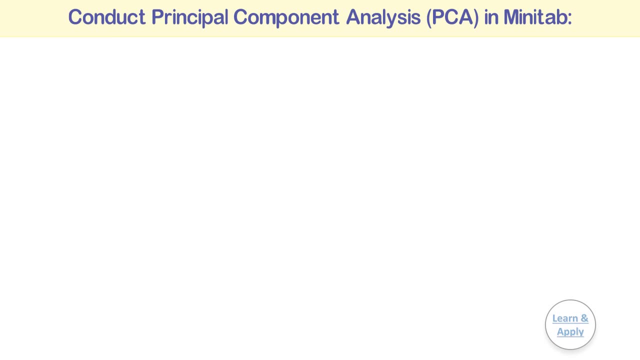 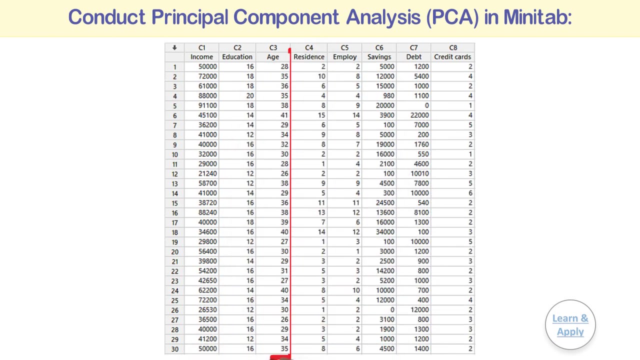 Conduct a principal component analysis in Minitab. To conduct a principal component analysis in Minitab, please follow these steps: 1. Enter or copy the data to Minitab worksheet with the data for one variable in one column, as shown in the picture. 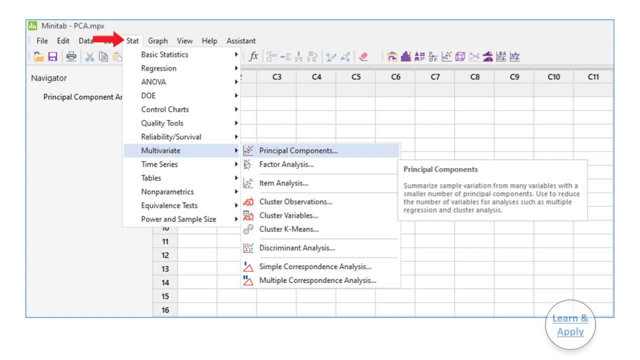 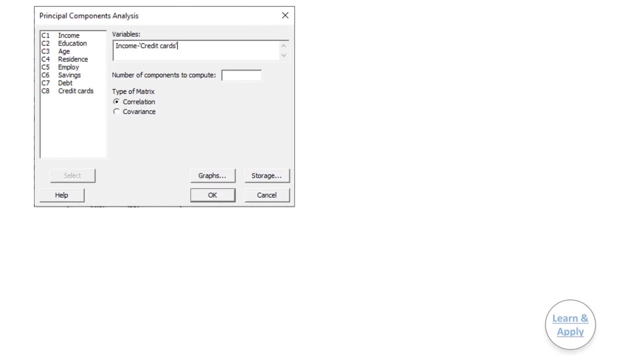 2. Select stat, multivariate and then principal components. 3. In variables enter c1 to c8.. 4. In the number of components to compute, keep the field blank. Here enter the number of principal components that you want Minitab to calculate. 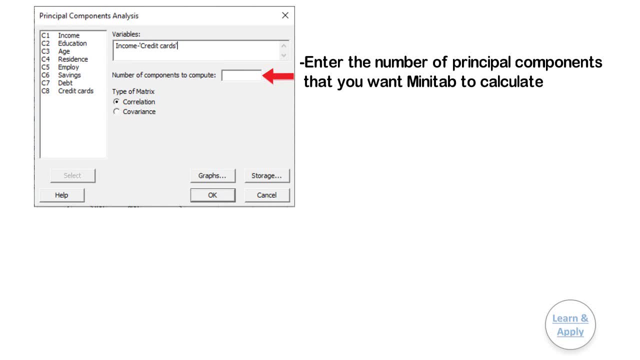 If you have a large number of variables, then you may want to specify a smaller number of components to reduce the amount of output. If you do not know how many components to enter, then you can leave this field as blank. 5. In type of matrix: keep the default selection of correlation as it is. 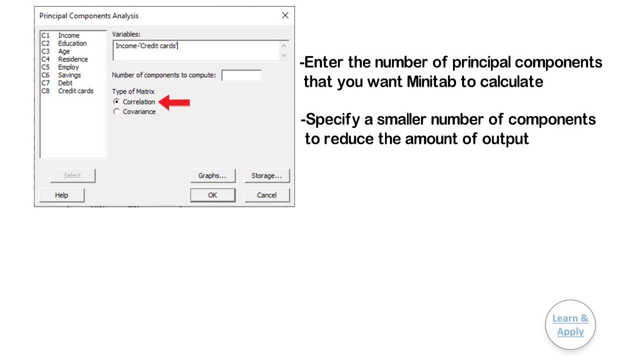 Here. please select the correct type of matrix to use to calculate the principal components. Correlation: This is used when your variables have different scales and you want to weight all the variables equally. Our example falls in this category: Covariance: This is used when your variables use the same scale or when your variables have different scales. 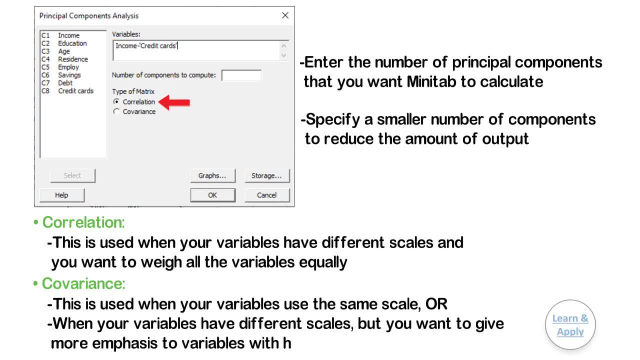 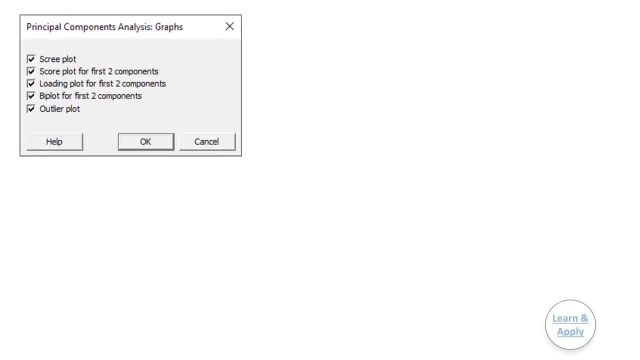 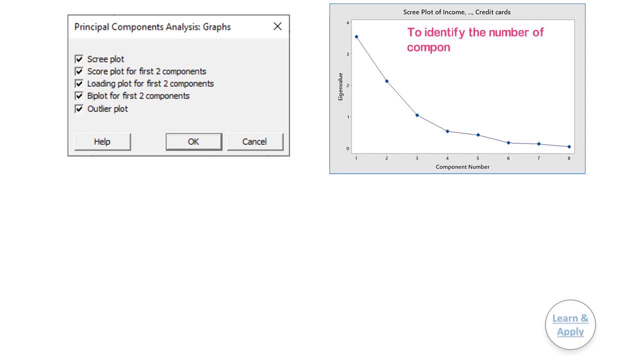 but you want to give more emphasis to variables with higher variances. 6. From the graph: select the graph you want to see for analysis. Scree plot. Use a scree plot to identify the number of components that explain the most of the variation in the data. 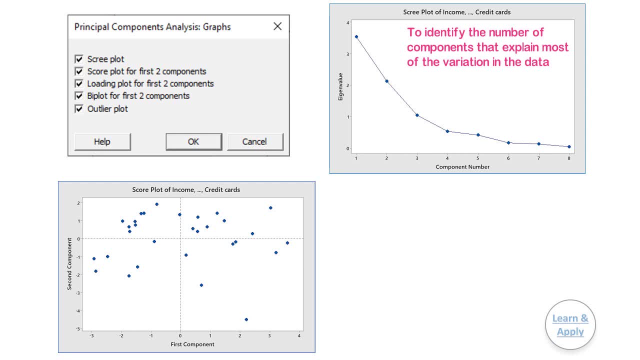 Score plot for the first two components. Use the score plot to look for clusters, trains and outliers. Use the score plot to look for clusters, trains and outliers. The then put the measurements in the first two principal components. Loading plot for the first two components. 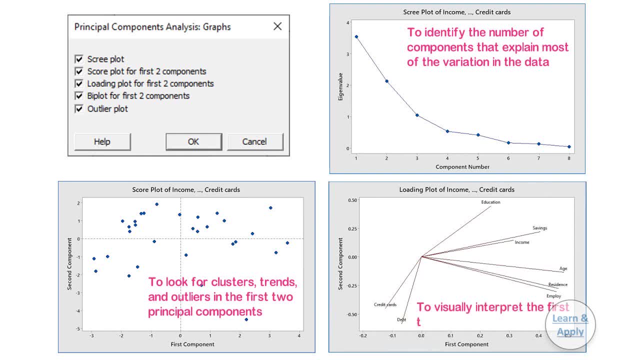 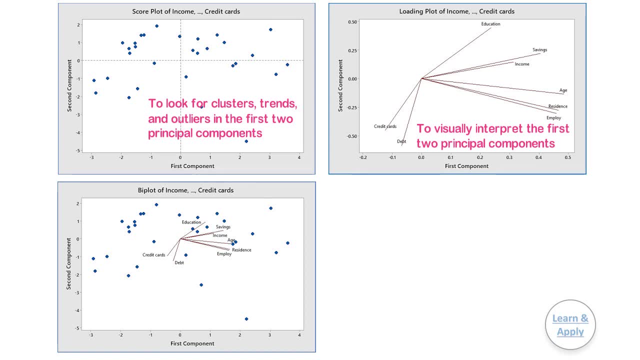 Use the loading plot to visually interpret the first two principal components. Byplot for the first two components. Use the byplot to look for clusters, trains and outliers. through the interpretation of the first two principal components. The byplot over lays the score plot and the loading plot on the same graph. 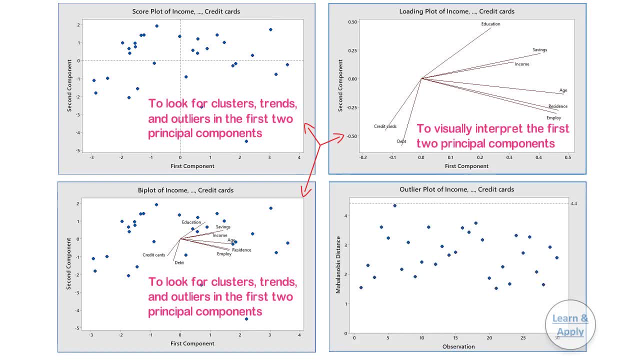 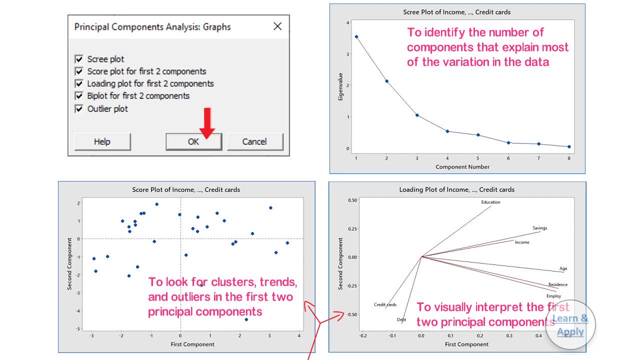 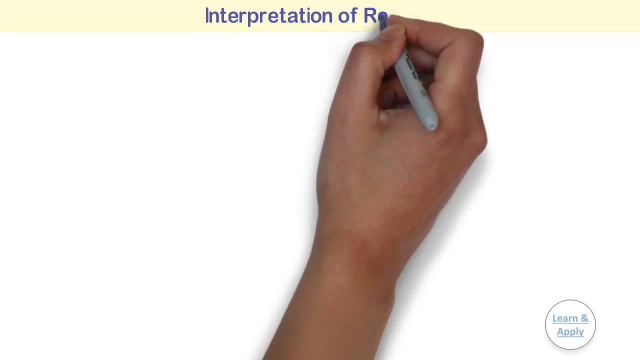 And Outlier Plot. Use the outlier plot to identify outliers in the data And 7. Click OK in each dialog box to get the results. We will get the results of analysis in the Session window and in Graph window. Interpretation of Results: In these results, use the cumulative proportion. 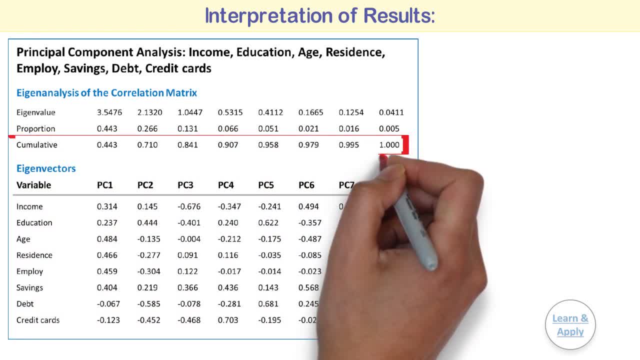 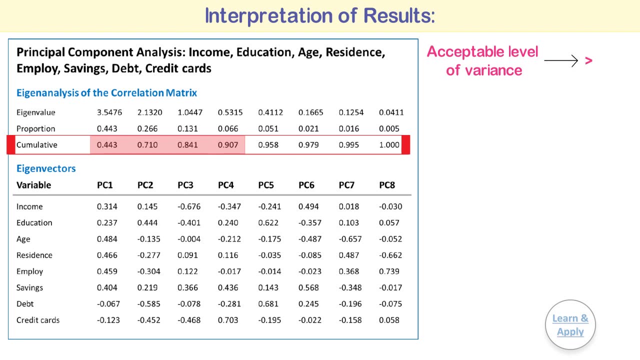 to determine the amount of variance that the principal components explain. Return the principal components that explain an acceptable level of variance. The acceptable level depends on your application. For descriptive purposes, you may only need 80% of the variance explained. However, if you want to perform other analysis on the data you may want to have. 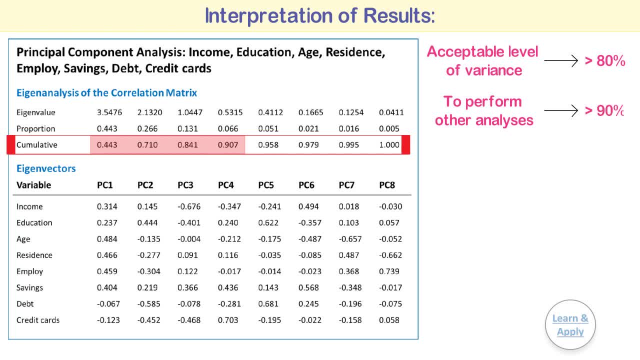 at least 90% of the variance explained by the principal components. This is the case in our example. The first four principal components are the principal components. The first four principal components are the principal components. The principal components explain 90.17% of the variation in the data. 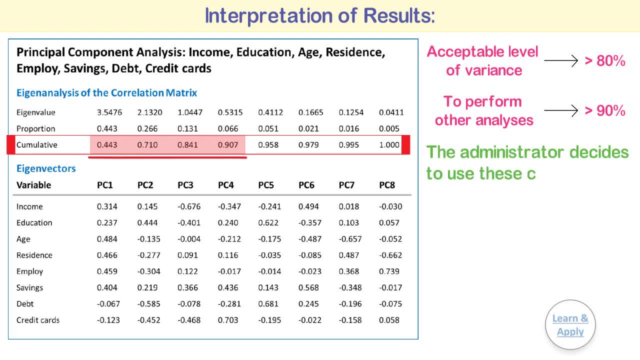 Therefore, the administrator decides to use these components to analyze the loan applicants. You can also use the size of the eigenvalue to determine the number of principal components. Retain the principal components with the largest eigenvalue, ie greater than 1.. 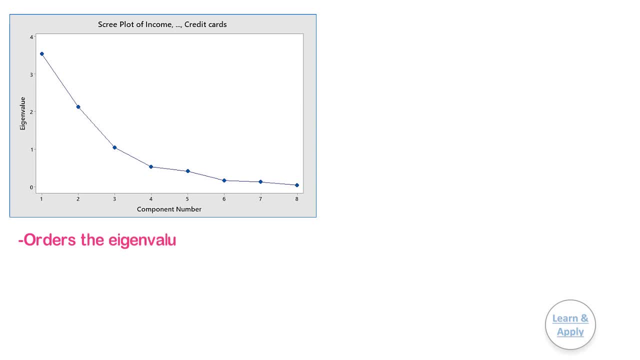 The script plot orders the eigenvalues from largest to smallest. The ideal pattern is a strip curve followed by a bend and then a straight line. Use the components in the strip curve before the point that starts the line trend. The loading plot visually shows the results for the first two components. 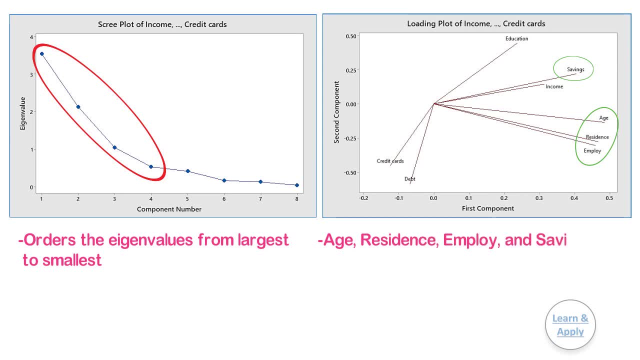 Age, residence, employee and savings have large positive loadings on component 1.. So this component measures long-term financial stability. So this component measures long-term financial stability. So this component measures long-term financial stability. The second: credit cards have large negative loadings on component 2.. 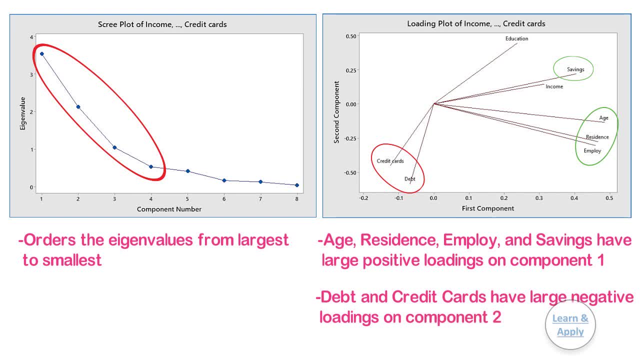 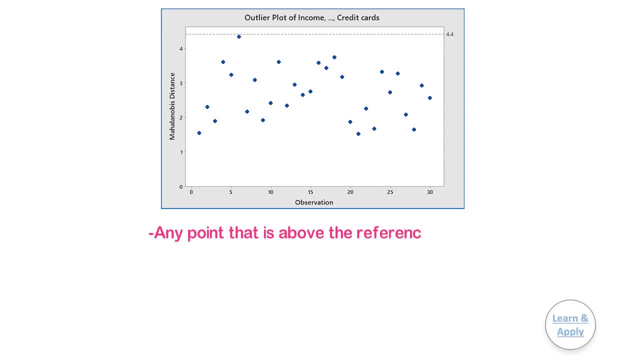 So this component primarily measures an applicant's credit history. Use the outlier plot to identify outliers. Any point that is above the reference line is an outlier. Outliers can significantly affect the results of your analysis. In these results there are no outliers. 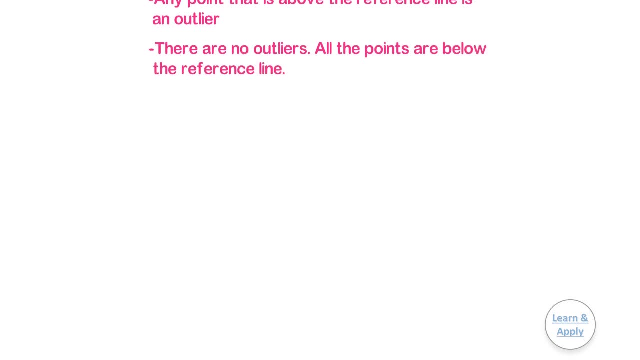 All the points are below the reference line. All the points are below the reference line. All the points are below the reference line. So objective-image waiting is an objective-image waiting. So, depending on the outcomes we get, we can make good records with our values. 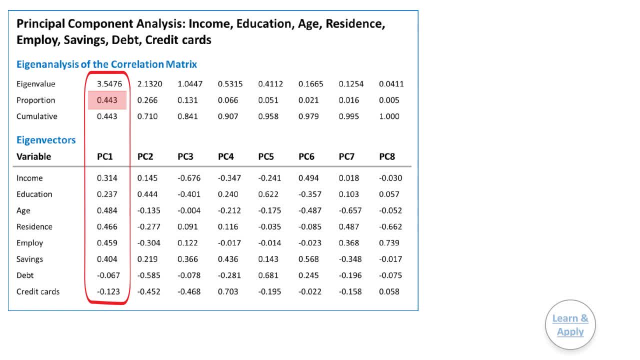 If any error occurs in the sample, an appropriate code may be used for information, And if an error occurs, we should cannot measure such a result. There are no tight tokens except There are no tight tokens except this: this, this, this. We used both the corresponding code. 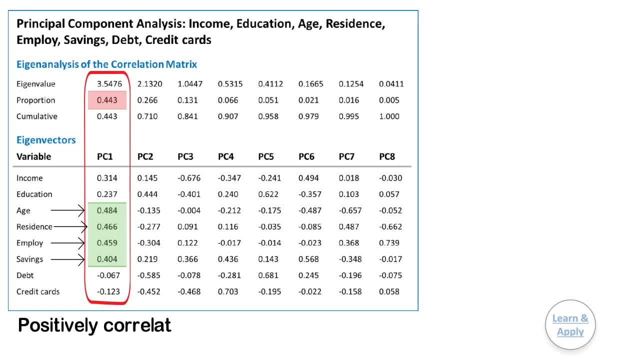 We used both the comparing code here. if a user wants a better score, write 2 characters from this part. you can also correct it for our results. age, residence, employ and savings increases the value of the first principal component. 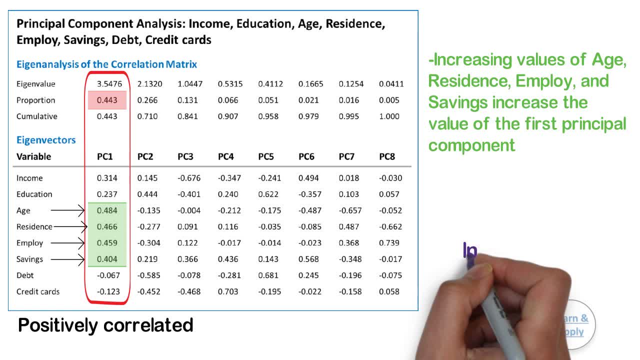 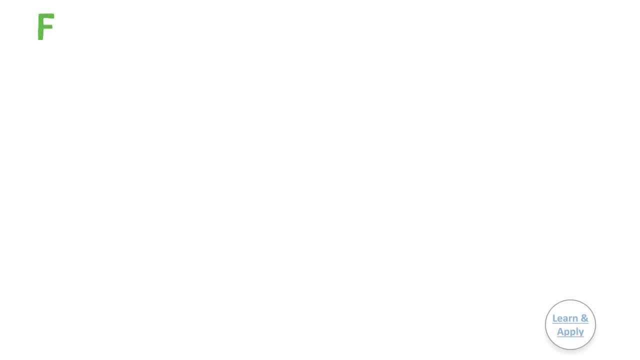 This is all about the detailed illustration of principal component analysis. We will see the next type of multivariate tools with a practical example in the next video. For references, I have taken some part of this very detailed content from Minitab Now to end. please like this video if you have found it useful. 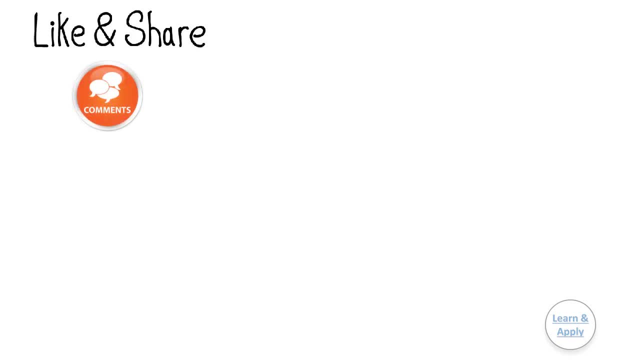 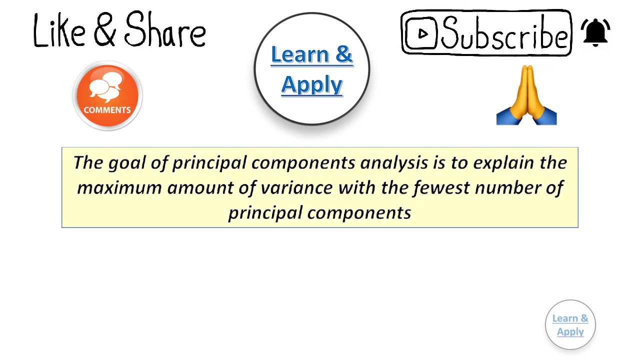 add your valuable comments and share this video to your friends and colleagues to improve and refresh their knowledge. If you want to get updates of such videos from my channel, please do not forget to subscribe it and click on the bell icon and select to get all notifications. And finally, thank you for watching. In this video you're going to learn how to transform parent functions, specifically parent functions that are in this form or this form. Now, a lot of times students get a little bit confused because they're not sure whether they do the horizontal shift first or the horizontal stretch. 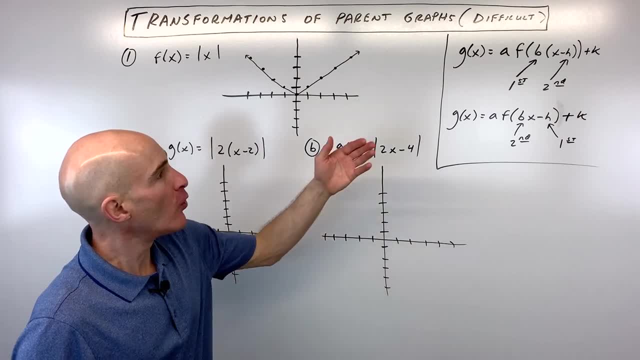 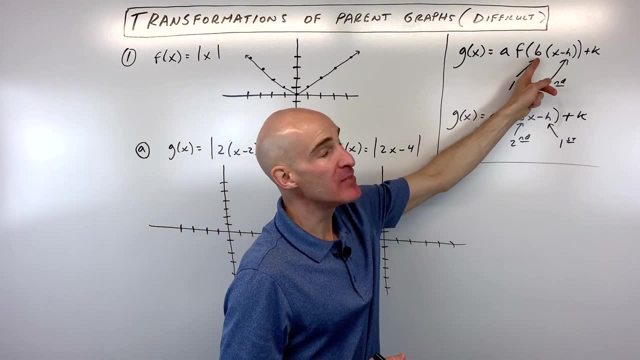 or compress first, and that's what we're going to clear up in this video. So when it's in this form here, where you can see the b value is factored out, what you want to do is you actually want to take the b into consideration first, meaning that you're going to either stretch horizontally 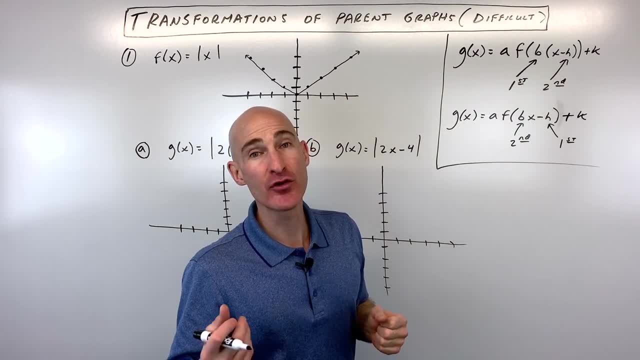 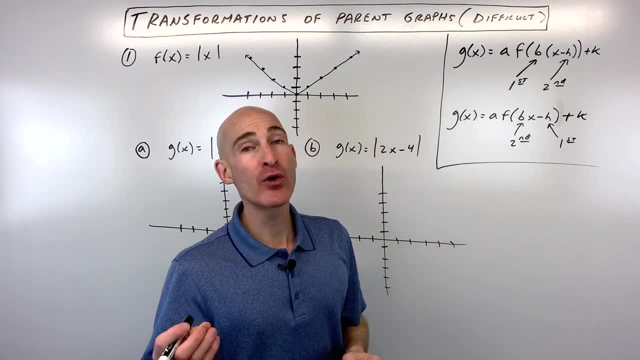 or compress horizontally the x coordinates of your graph, and then you're going to follow that up by shifting it left or right, And that's what the h indicates here. Now, the important thing to remember is that the number grouped with the x- okay in both cases- here the b and the h are.